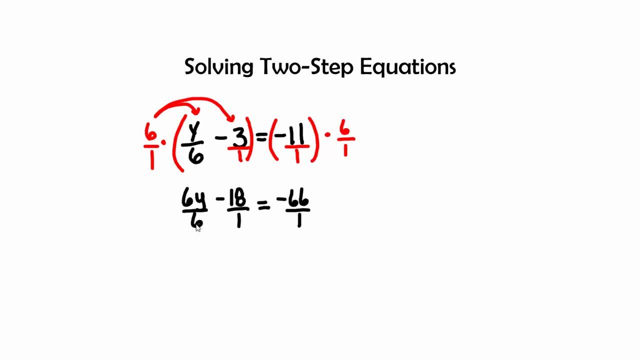 of the fractions. So let's start simplifying. 6 over 6 is 1.. So I have y by itself Minus. 18 over 1 is just a negative 18.. Equals negative. 66 over 1 is a negative 66.. 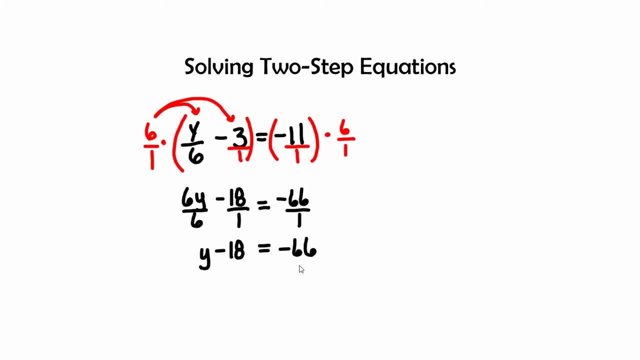 Now this looks a lot better. No more fractions. We got rid of the fractions. Let's just do our one-step equation. Here we have negative 18.. To get rid of that, I'm going to have to add its inverse, So positive 18 to both sides. 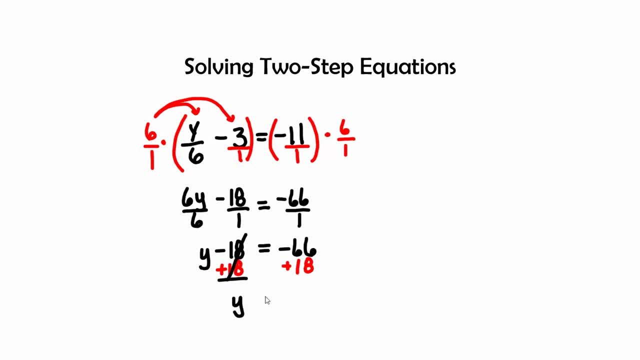 This is going to create a 0,, leaving y by itself, And then a negative 66 and a positive 18.. Some of you guys might be you might freak out, because this is not necessarily a familiar number, But which number has the most negative signs or positive signs? The 66 has the most negative signs. There's 66. 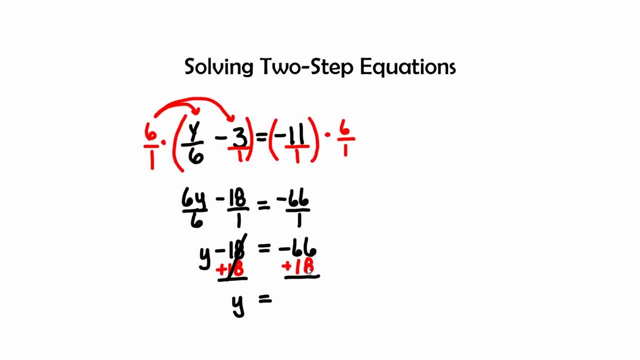 negative signs here And there's only 18 positive signs, So there's more. My answer is going to have a negative. I'm going to have more negatives than I do positives, So 66 and 18 is going to. we're going to subtract those two numbers from each other. 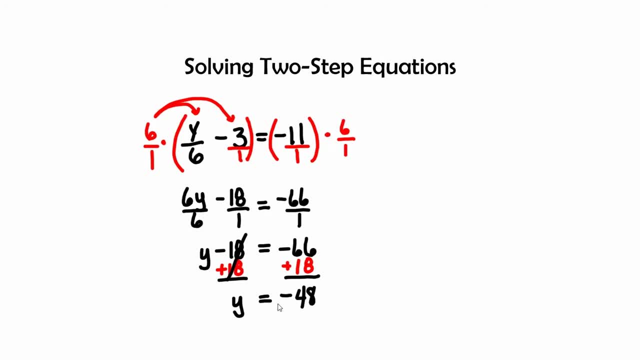 We're going to get 48. So our answer is: y equals a negative 48.. Now let's go ahead and plug it in. So wherever I see a variable, we are going to check our answer. So wherever I see a variable y, I'm going to put parentheses over. 6 minus 3 equals a negative 11.. 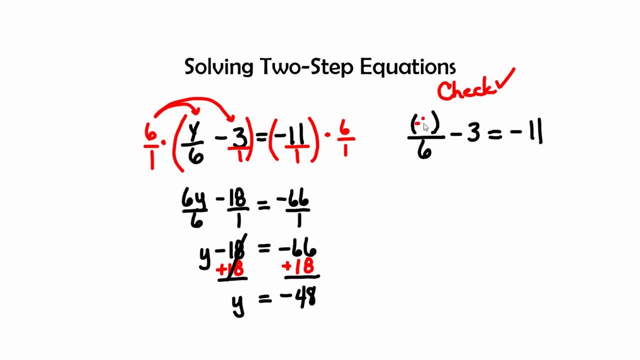 When I plug in the negative 48, negative 48 divided by 6 is a negative 8 minus 3 equals a negative 11.. Negative 8 and a negative 3, we combine those together gives me a negative 11 equals a negative 11.. And we check, So don't.